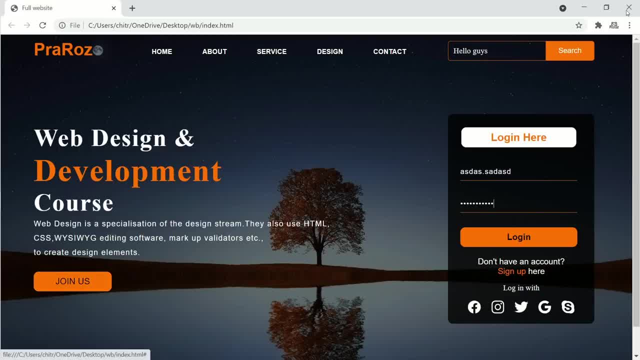 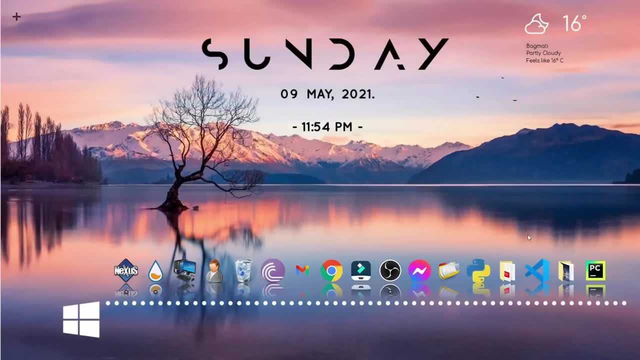 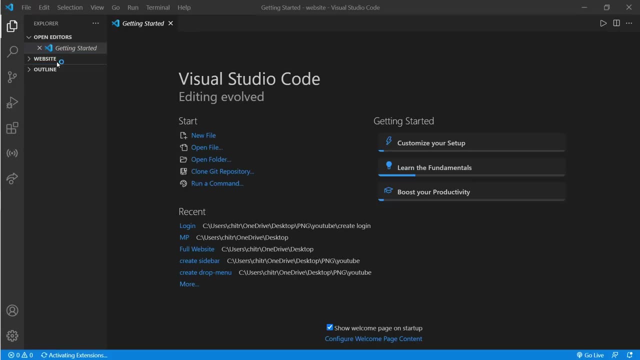 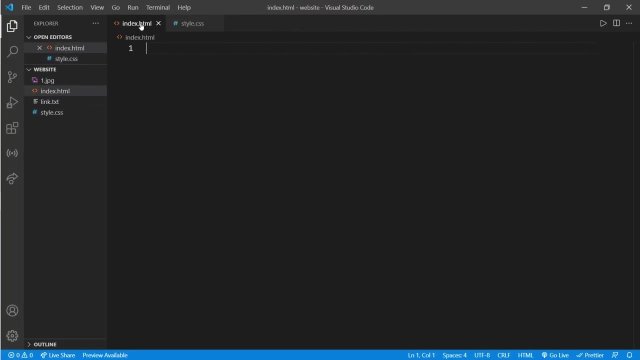 everyone can understand, including beginners, very easily. okay, I have a folder named a website and a background image. open a VSCode and select a folder which you have created and create a file named indexhtml and stylecss. okay, and click on class chant and delete this. we don't need it. 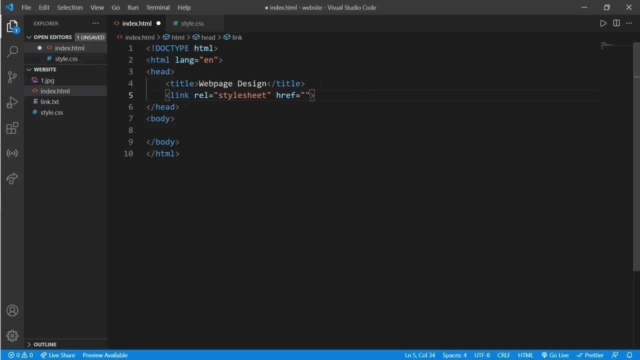 I would name my website a website design and link this webhg with stylecss. okay, inside the body we create a div, dot main, and inside the class MN we create another div, that's napbar. we create dot icon, which is for our logo, class logo and then P R A R O Z. 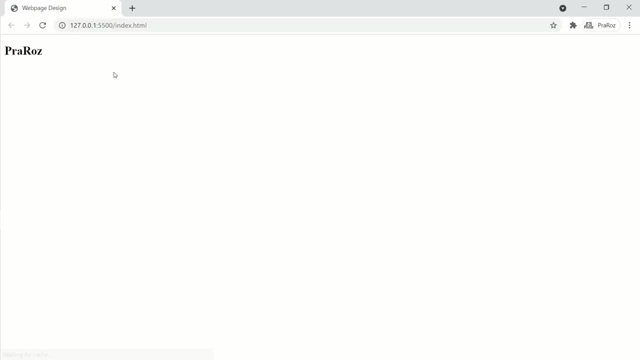 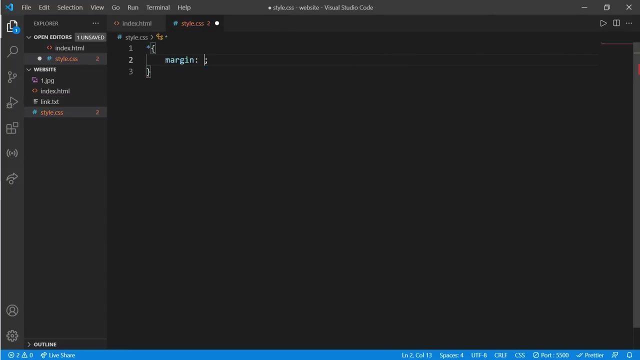 let's see in the browser. ok, here we have our logo. we go to stylecss, put a margin of zero, padding also zero. we go to our classmain with the hundred percent background linear gradient making our background image 50% dimmer. connecting with URL 1.jpg. 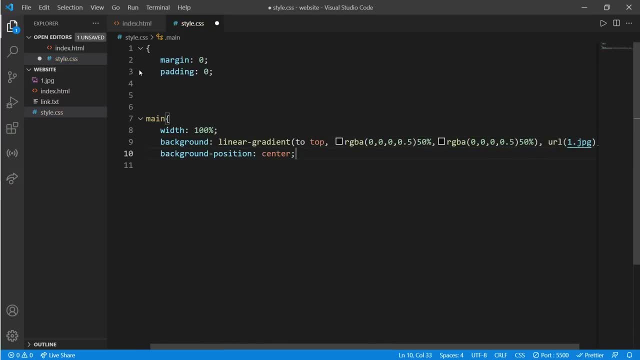 background. position of center and background size, cover and height of 100 ways. you go back to our website and see it looks good. now let's go back to next class navbar. width of 1200 pixel. height of 75 pixel. margin: auto. go to next dot icon with 200 pixel. 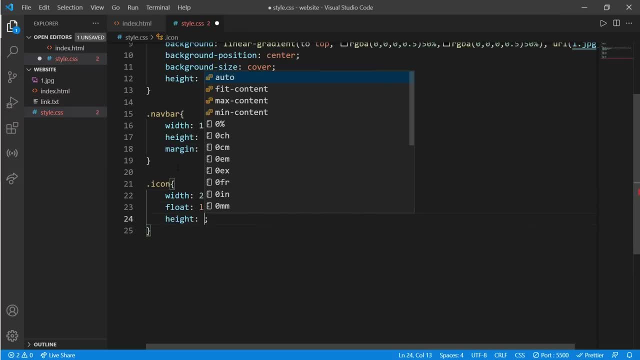 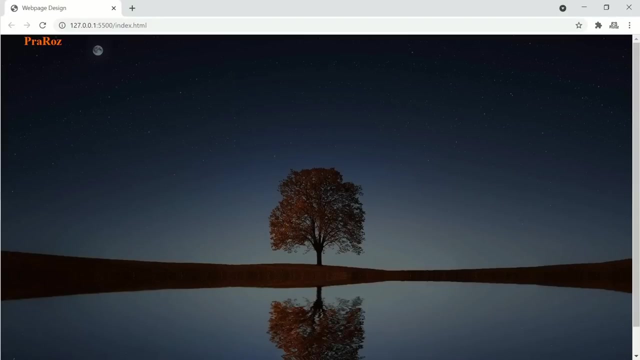 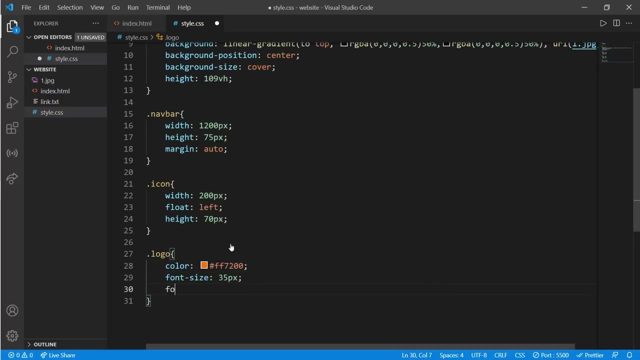 left height 70 pixel and go to dot logo and will keep color like orange color, let's see in website. ok, looks good. now on font size of 35px, font family arial, padding left: 20px, float left and padding top: 10px. 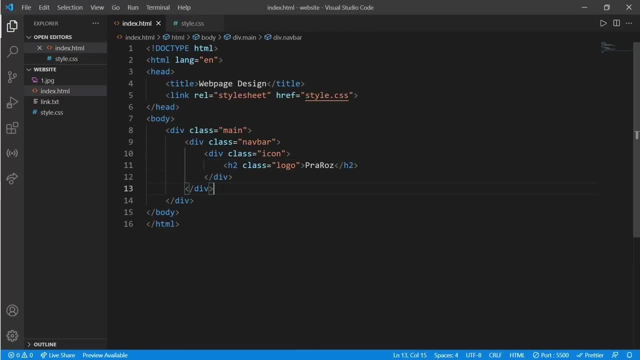 Now we go back to index and create another div- that is for menu, that is divmenu- and create another list inside another list. we create a list and anchor tag and we copy this and paste and type a home about service design and a contact. 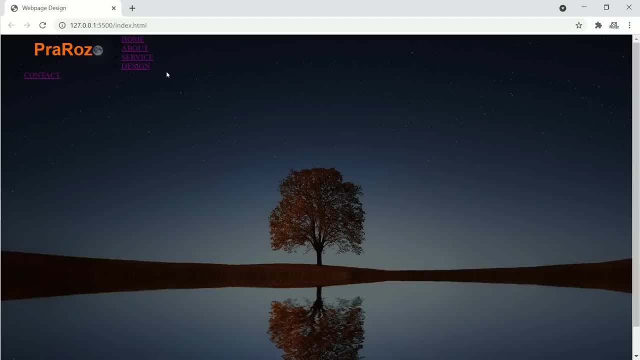 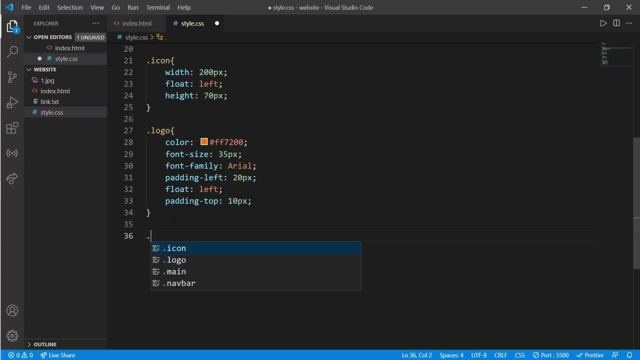 Now let's go back to our website. ok, here we have our menu. go back to stylecss dot menu. ok, here we have width of 400px and float left and height of 70px. ok, it looks good. ok, now we go to another list. float left, display, flex and justify content center and. 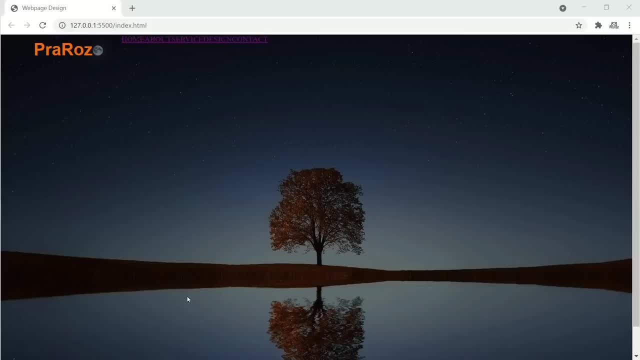 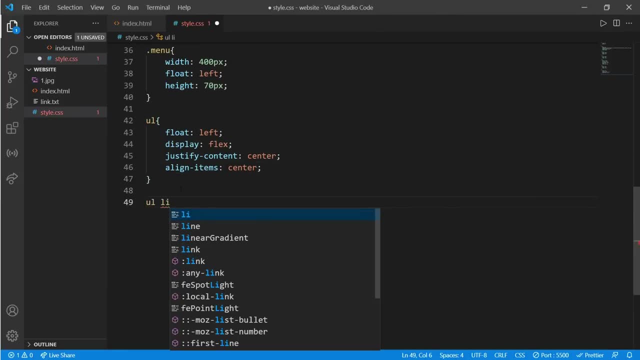 align item also center. ok, let's go to our web page and here we have: ok. now we go to another list inside list and we have list type: none and margin left and height of 70px. ok, Ok. Margin top: 62px, margin top 27px and font size: 14px. ok, now it looks more good, ok. 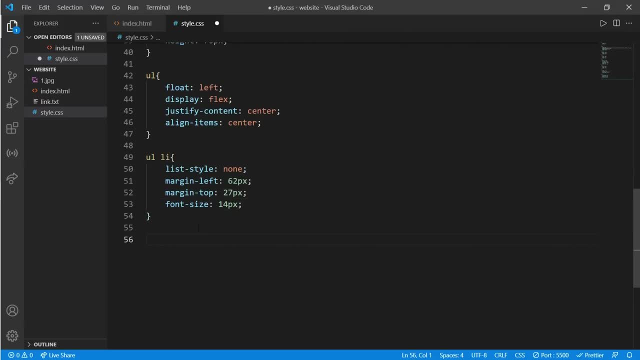 now we go to another list list anchor tab, which is text decoration color white. ok, ok, Ok, Ok, Ok. We will put cont现在titling and image of text value agora, Ok, Ok, nowcrire, and we will keep marrying text. 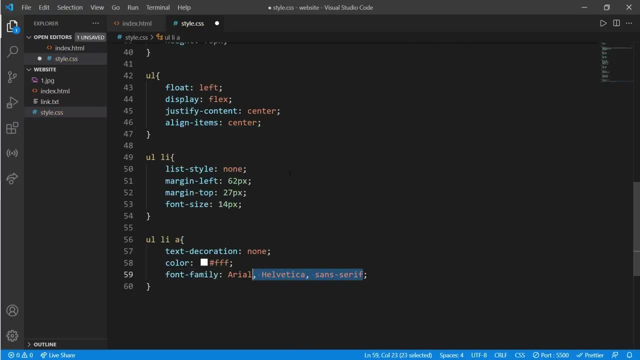 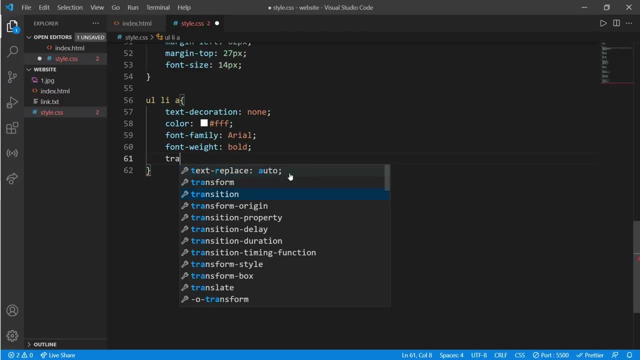 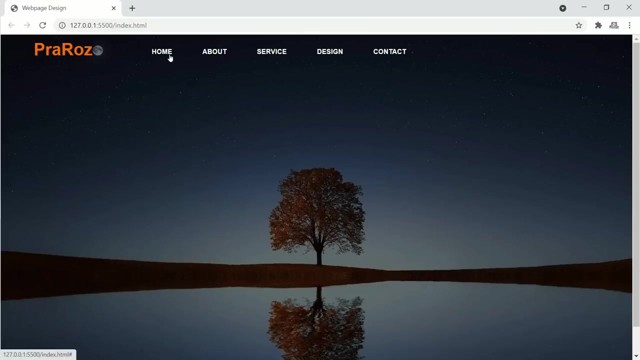 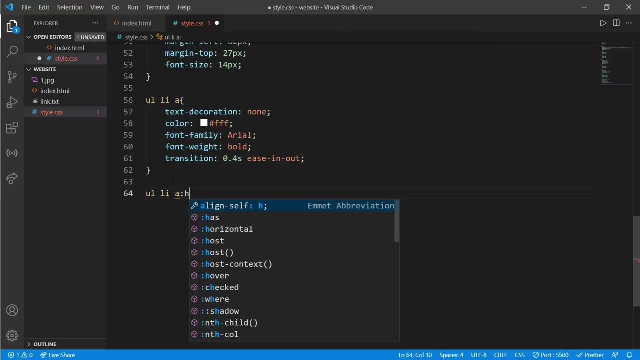 and text type 3 and font family aerial, and font width bold, and we have transition of 0.4s is out. Ok, now we will put a hover effect in our helps. and now let's Agree to her monkae MODE color. 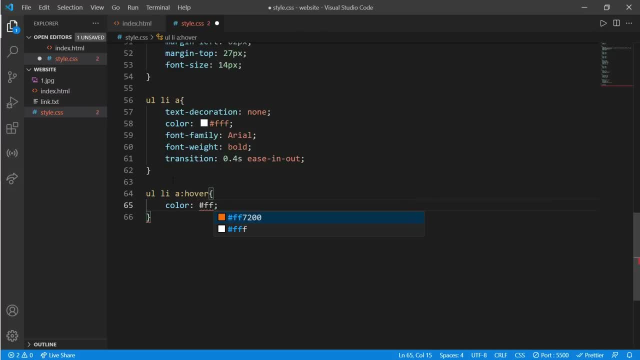 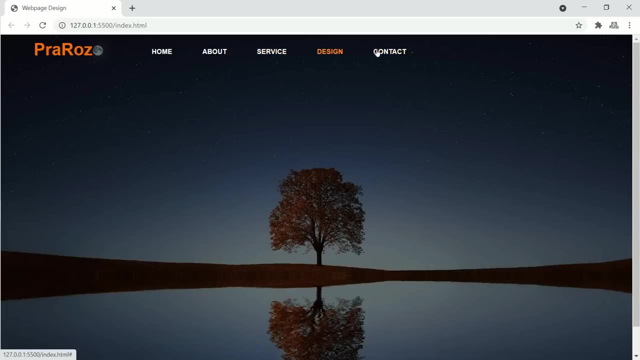 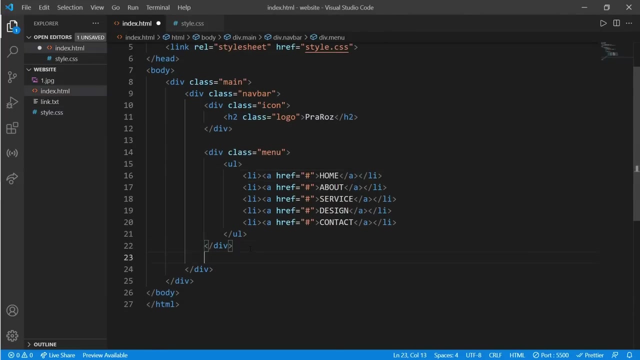 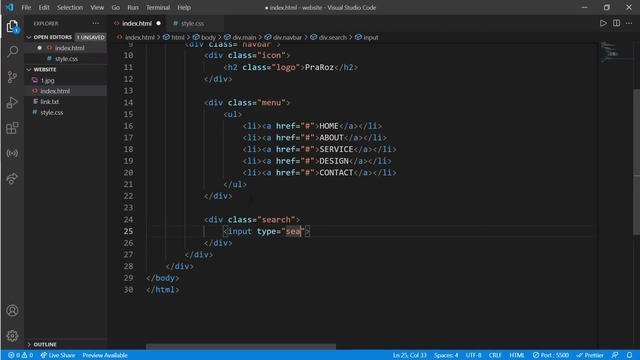 video orange. okay, here we have our hover effect on our menu bar. now let's get back to our index and create another dip. that is for search bar. we put input, it is for search name, placeholder, type to text and class, srch. okay, anchor tab button. inside button we put a class, that is BTN, and another search. okay, here we have our. 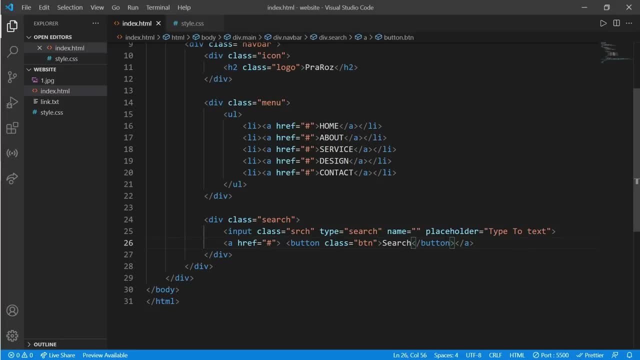 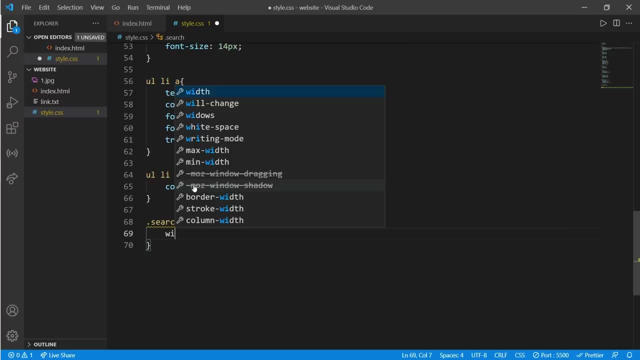 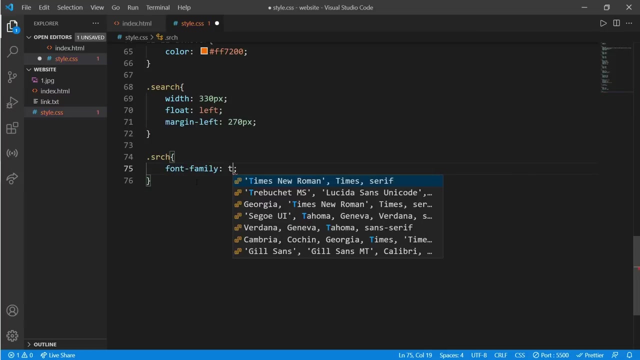 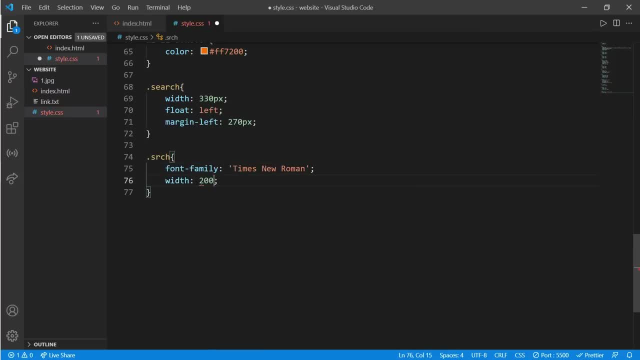 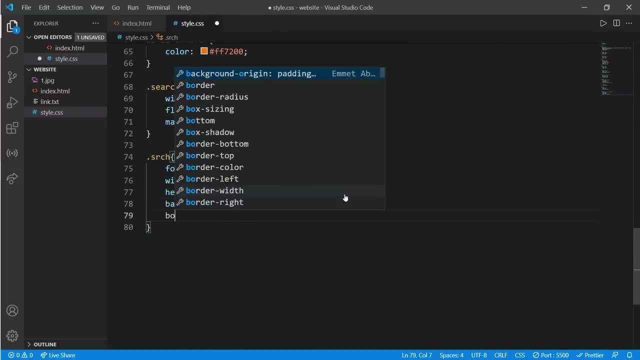 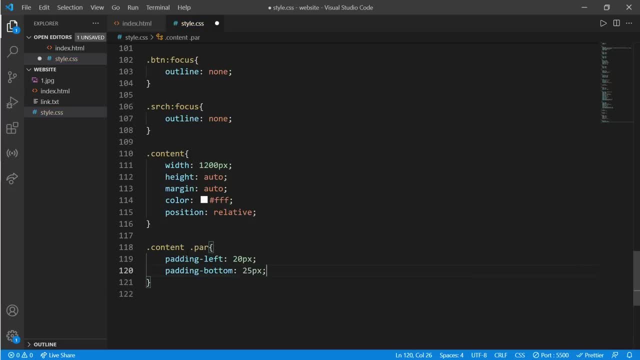 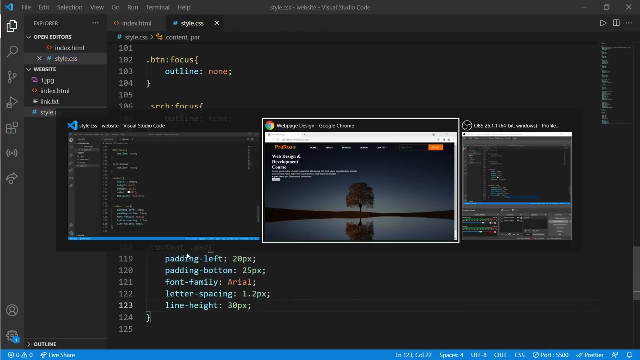 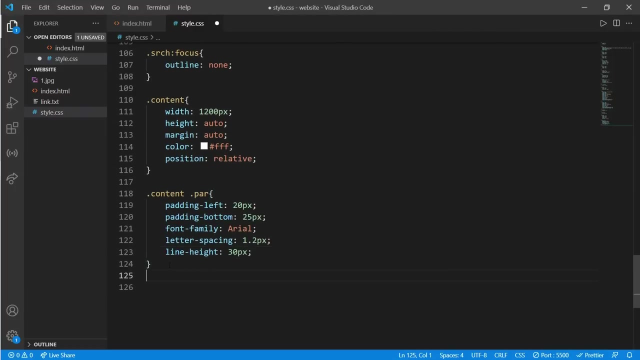 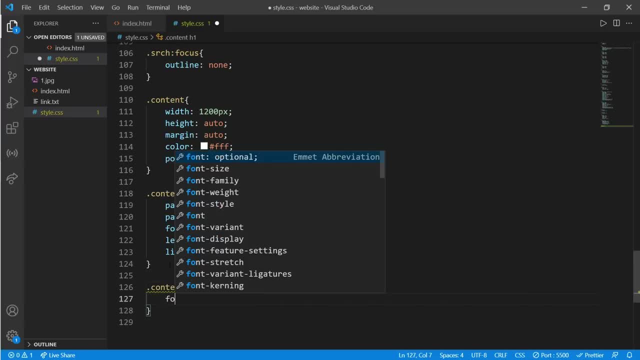 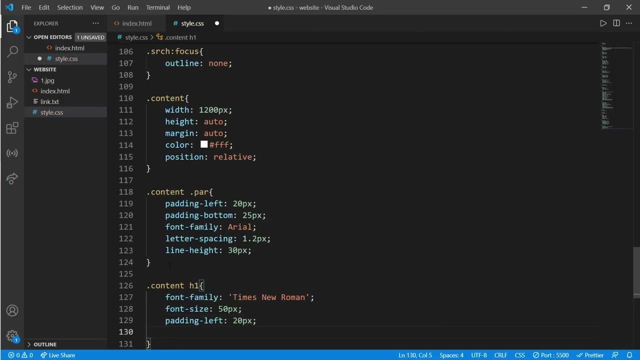 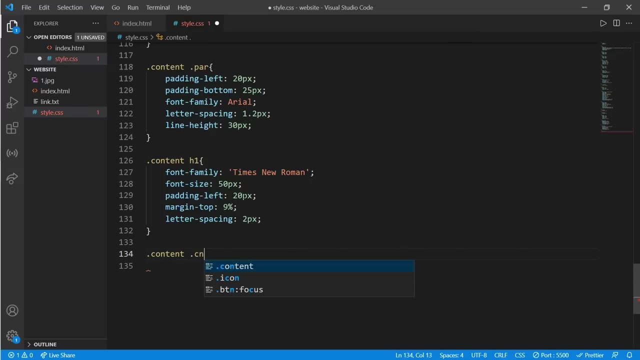 that's one tag, yeah, one family of times. new roman font size of 50 pixel. padding left would be 50 pixel, 20 pixel margin, top 9% letter spacing: 2 pixel. okay, more better, then we will add that content for that contact, that is of join us with 160. 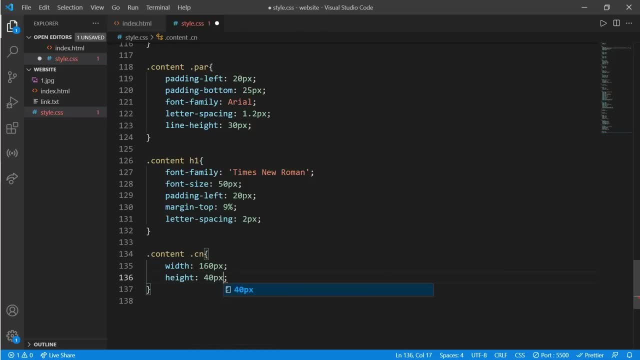 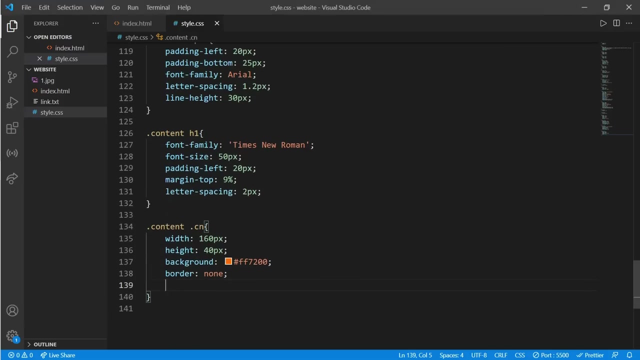 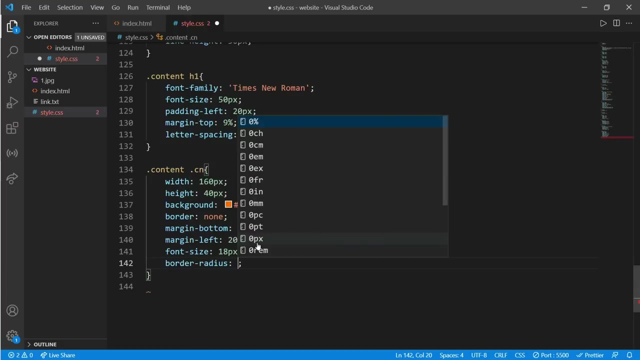 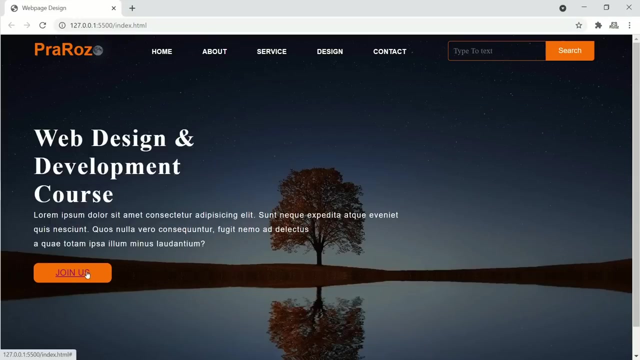 pixel height of 40 pixel and background orange border. none, here is our link. join us. and we put now margin: bottom of 10 pixels, margin depth: 20 pixel. okay now. font size: 18 pixel. border radius of 10 pixel and cursor point pointer: okay, it looks good. now we need to remove that underline. so we go to next class. 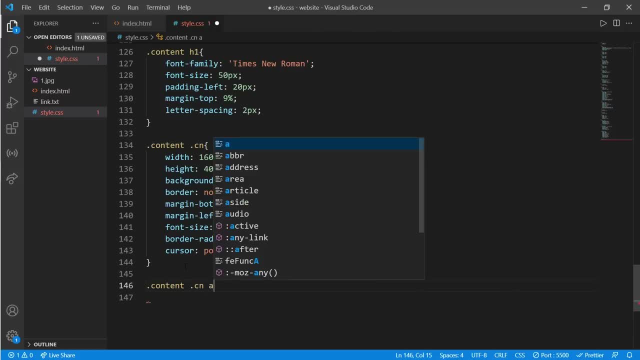 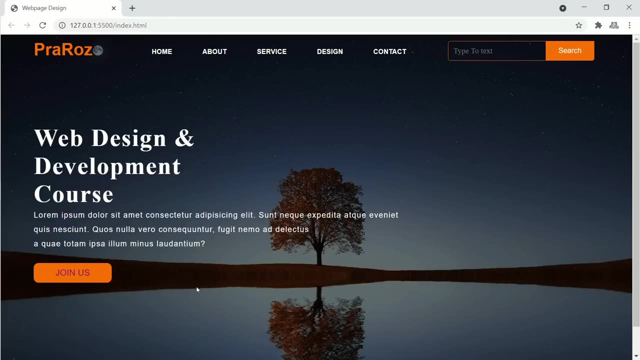 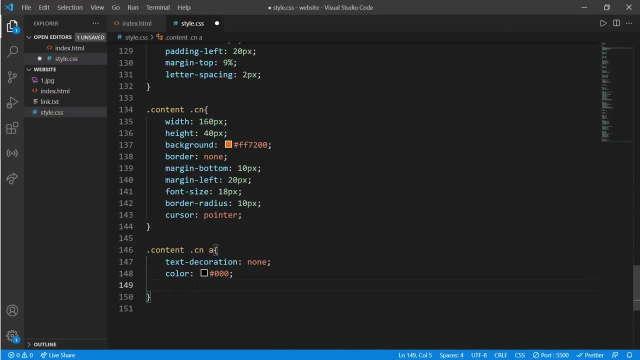 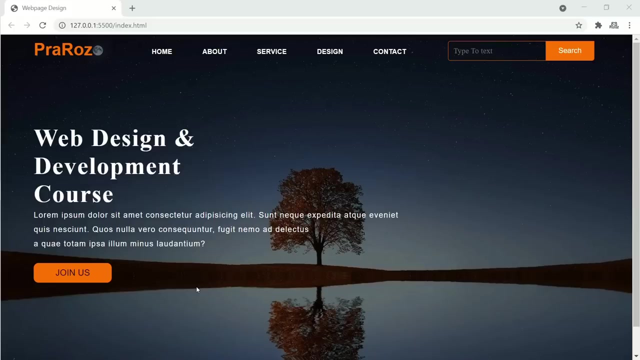 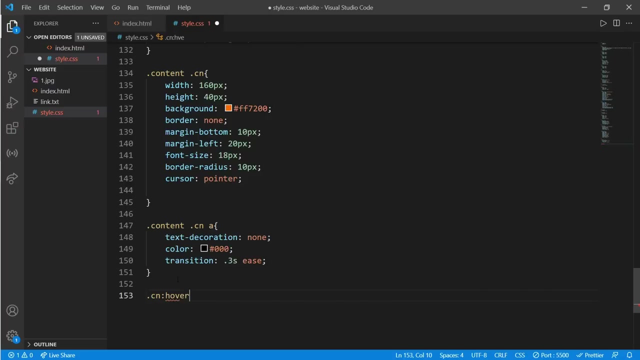 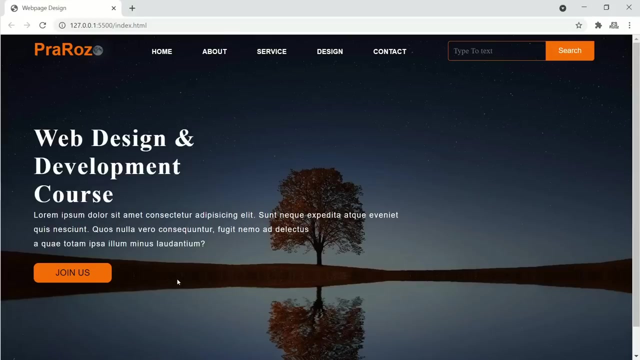 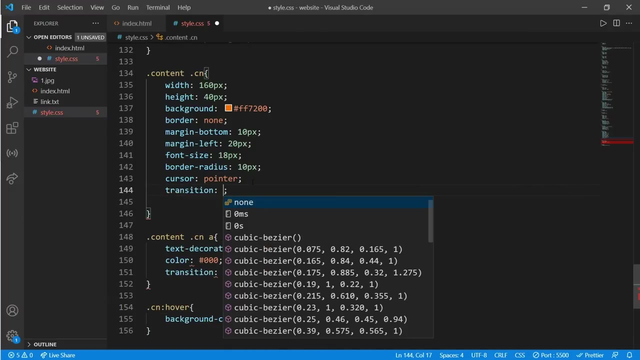 content: dot CNE and we'll text decoration: none. okay. now color: put a color of black and transition would be 0.3 is and we'll put a hover effect in over there. background would be white. okay, now put transition time: 0.4 years is okay. now it looks more good. 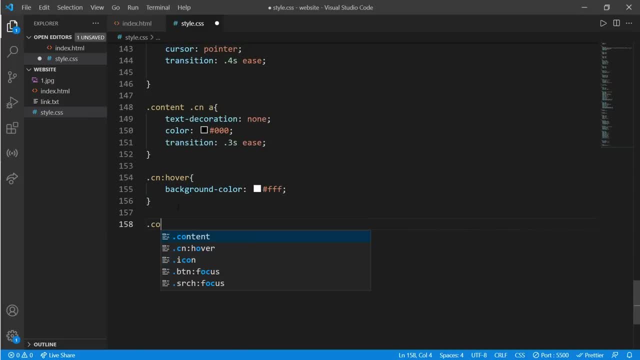 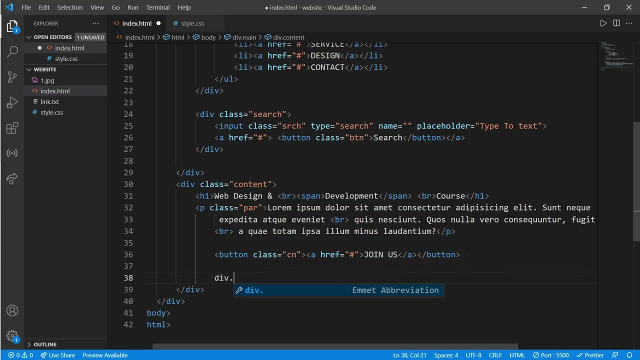 now content, dot content for a span that is inside depth for development. we put orange color and font size of 60p, 60 pixel. okay, now we get back to index dot HTML and create another div, that is for our login box, this deep, dirt form and h2 tag. login here and put. 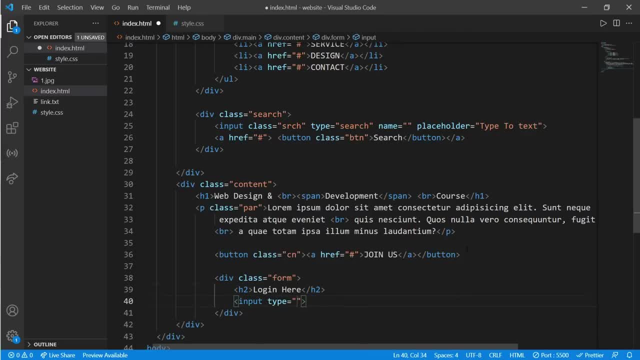 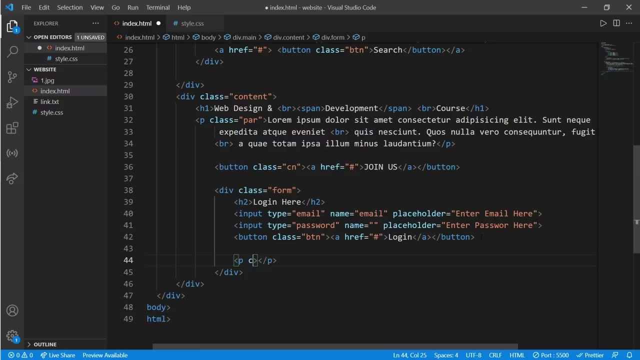 an input type email name: email and placeholder: enter email here. and input for password type password: placeholder: enter password here. then button class: BTNN. anchor tag here: login. okay, here we have our login box now in paragraph tag be class link: I don't have an account and break anchor tag: sign up here. 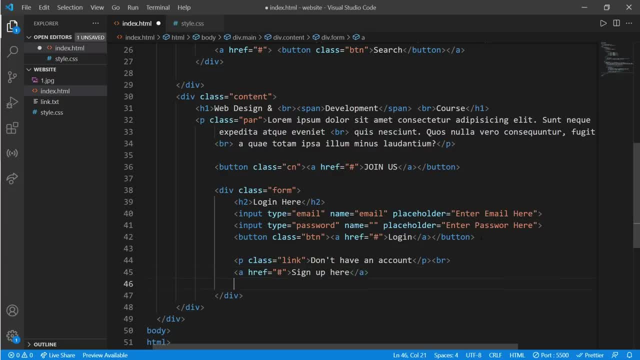 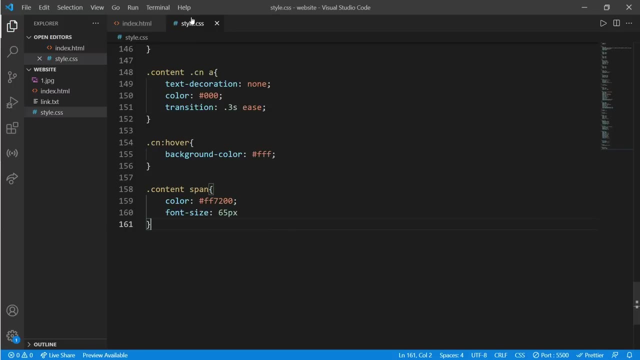 okay, now again p tag class login: width: okay, and we'll move it to right. go back to stylecss. start from now, width would be 250 pixel. height would be 380 pixel. background linear gradient: okay. here says, in terms of section width, to go forward like this: then, mr p option. 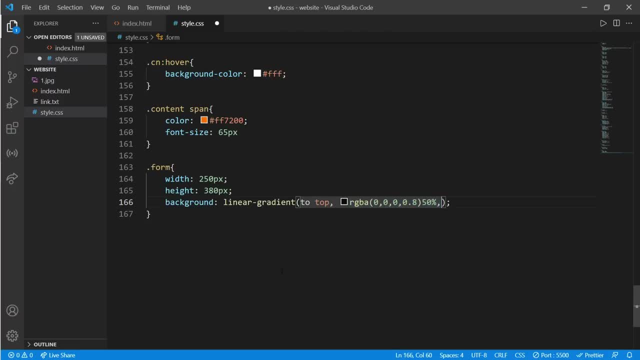 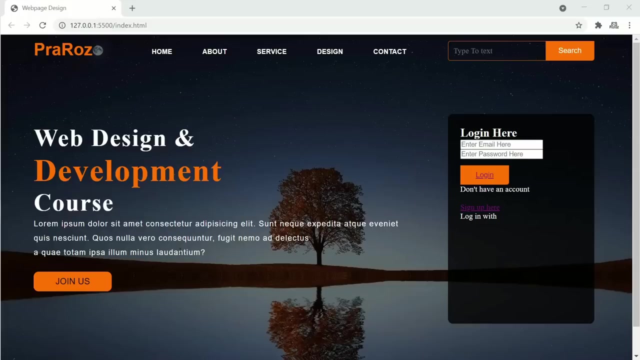 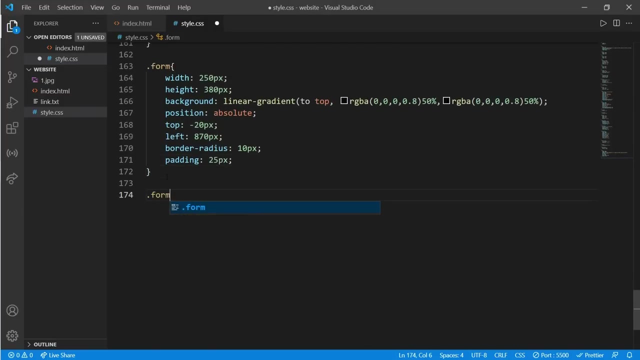 paste to have minimum pend gun sparse right to top, just like before, and then Susan would be absolute and top would be minus 20 pixel and lift 870 pixel. okay, it looks more good. now we'll add our airport flat map: radius of 10 pixel and padding: 25 pixel. okay, more good then. h2 tag width of 220. 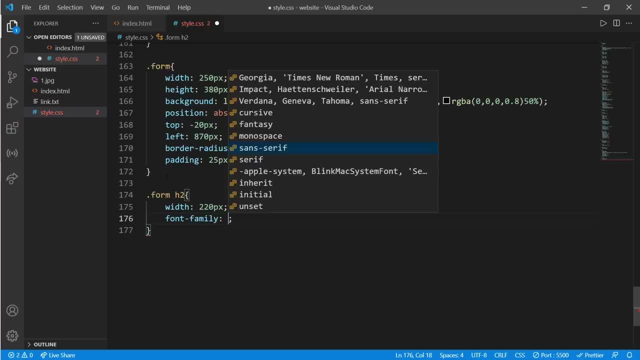 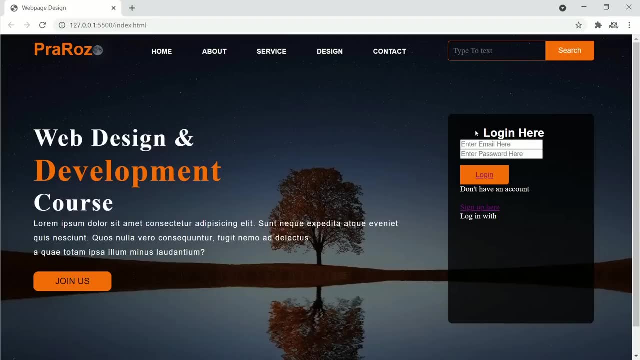 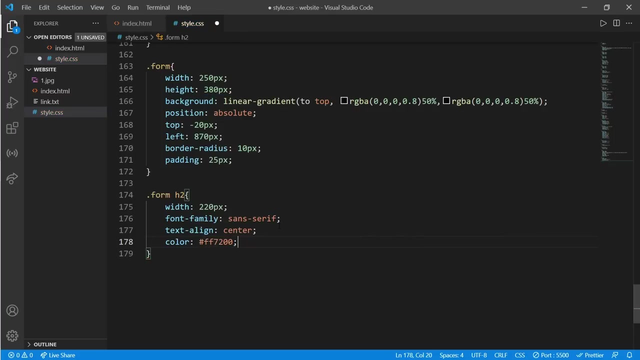 pixel. font size: font family: sans-serif text align center: okay, and color would be orange. font size: 22 pixel. background color: white: you, and border border radius would be 10 pixel. margin: 2 pixel. padding: 8 pixel: okay. okay, now for dot form input. I will pick width of 240 pixel and a height of 35. 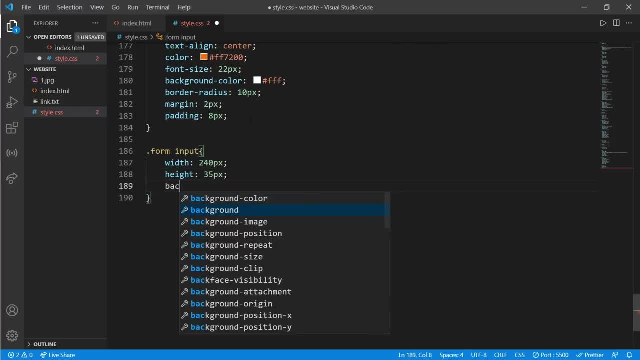 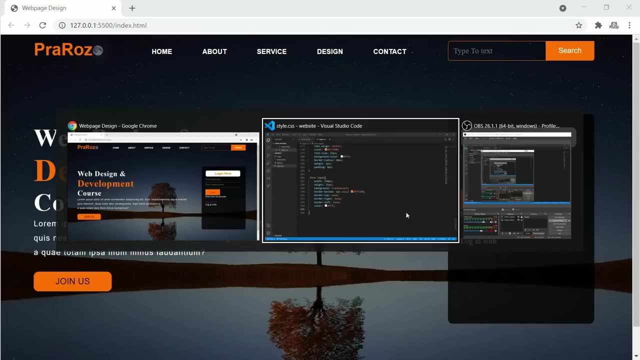 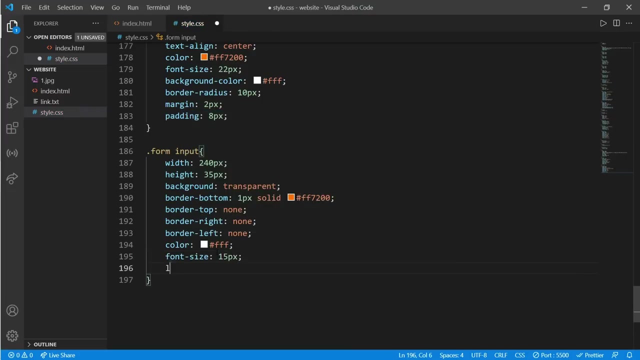 pixel, 16 pixel and border-left also none and we'll have our color white. okay, it looks more good. and font size of 15 pixel and letter spacing would be 1 pixel and margin top 30 pixel. font size or font family would be sans-serif. 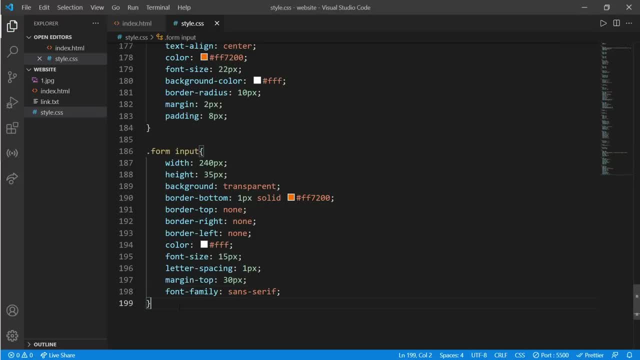 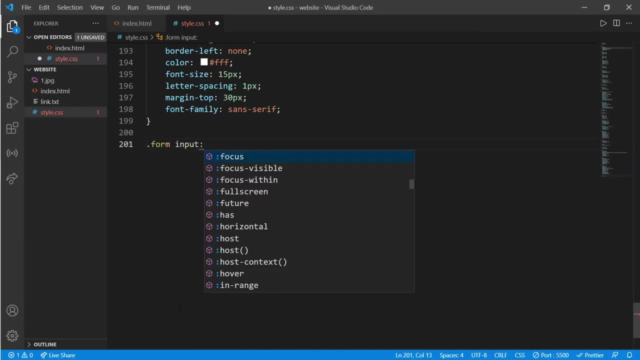 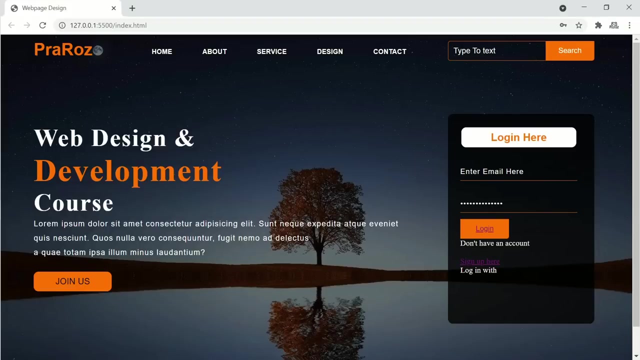 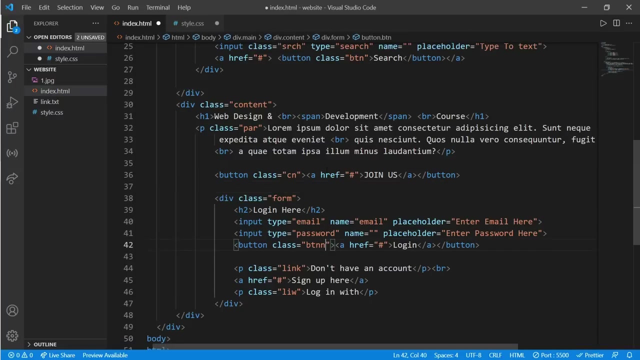 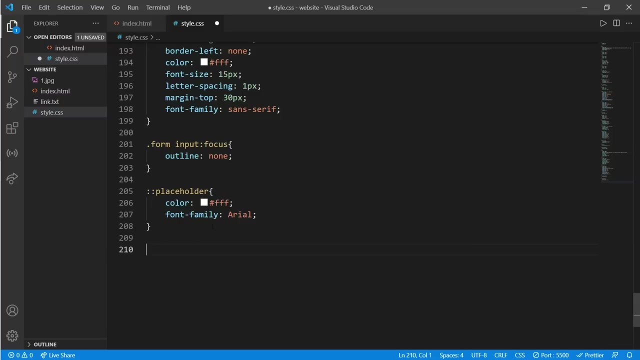 okay. okay, now we'll have draft form, input, focus and outline none, and for the place folder we'll have a color, white and font. family of Arial. okay, it is more brightened and darker now. okay, now we go, and here I have made a mistake: dot P T N? N, that is. 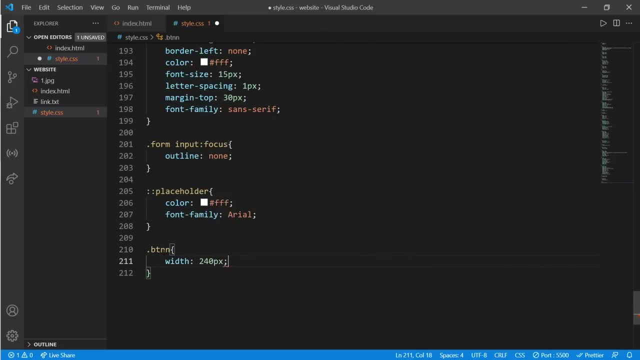 width of 240 pixel and the height of 40 pixel, and background will be orange. okay, here is our login box, and then we keep our border none. margin top would be 30 pixel, font size would be 18 pixel and border radius would be 10 pixel. 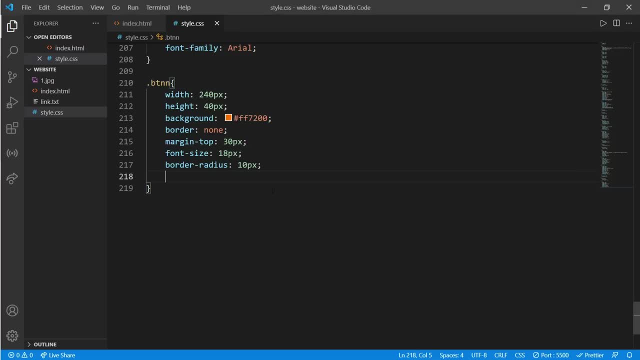 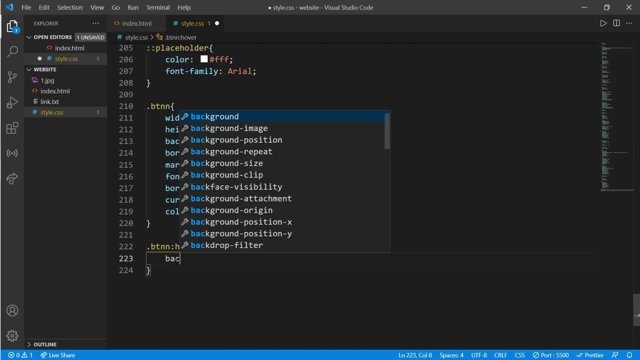 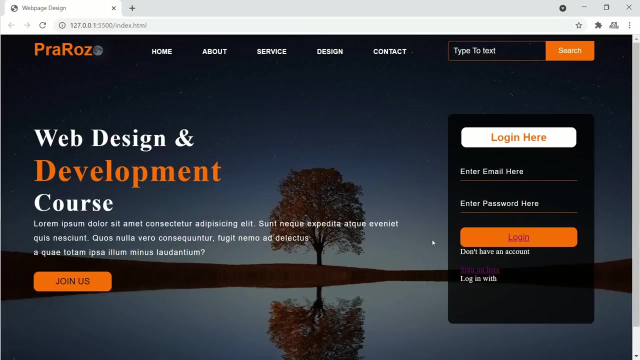 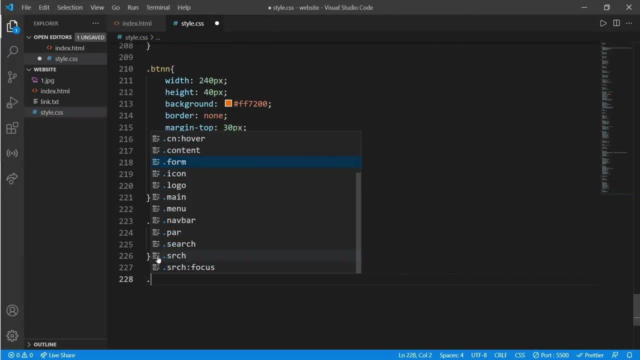 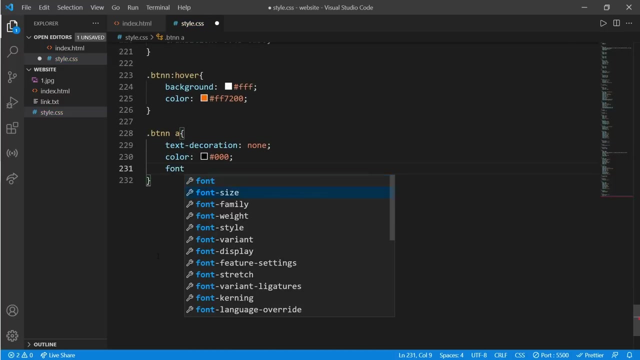 okay, it looks more good, and cursor would be pointer white. now we'll put a hover and background would be white and color would be orange. okay, remove a text decoration. remove that line with the text decoration: btnn. a text decoration: none, and color black: okay, and a font weight would be bold. you know, it looks more good. 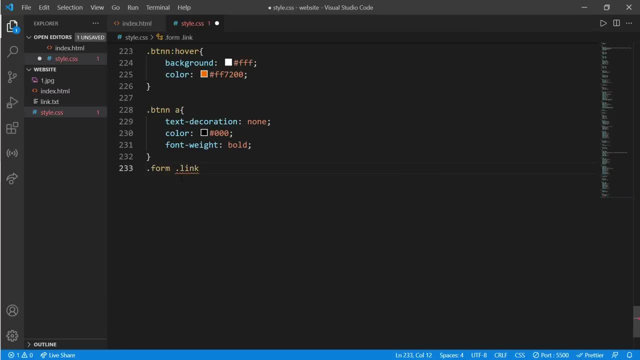 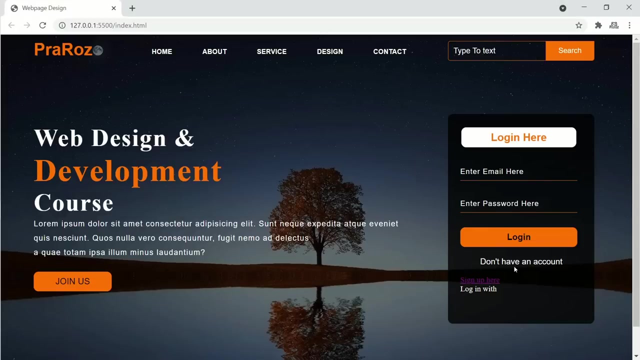 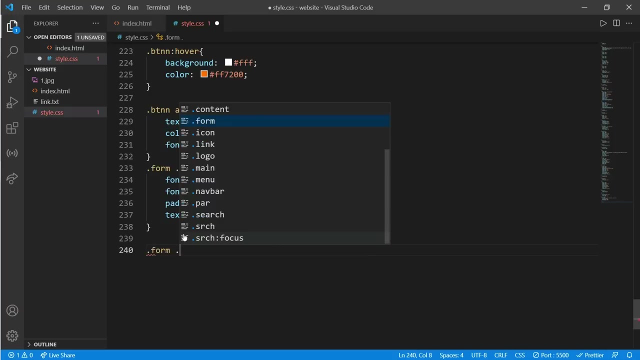 now for from that link. keep our font family area and font size of 17 pixel. padding top would be 20 pixel and text align would be Center, okay. okay, now we'll have dirt firm dot link, anchor tag link, anchor time and have text decoration of none and color orange, okay. 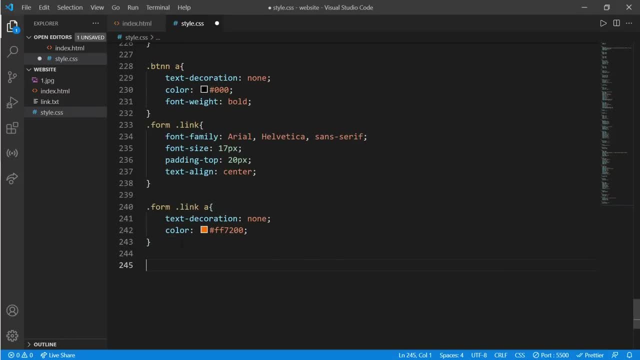 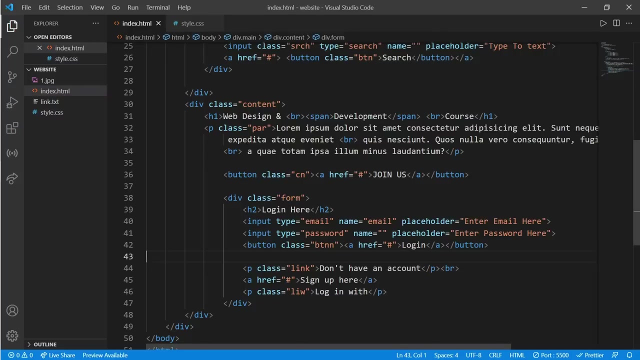 hmm, now I'm a login with a text decoration of none and color orange. okay, now I'm a login with a text decoration of none and color orange. okay, in with padding top of 15 pixel and padding bottom 10 pixel, and text align would be Center. okay, now this sign up here is not working. wait, okay, my. 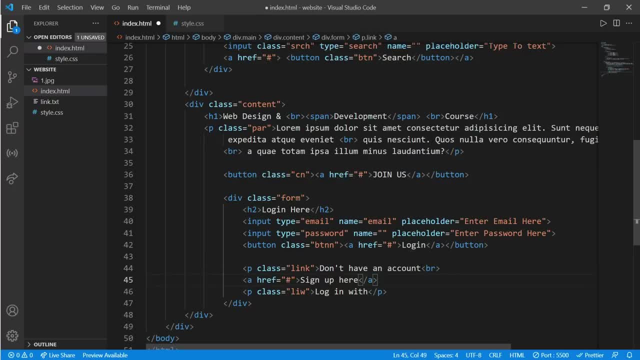 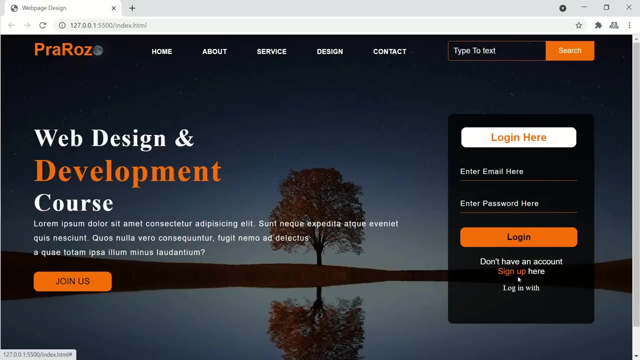 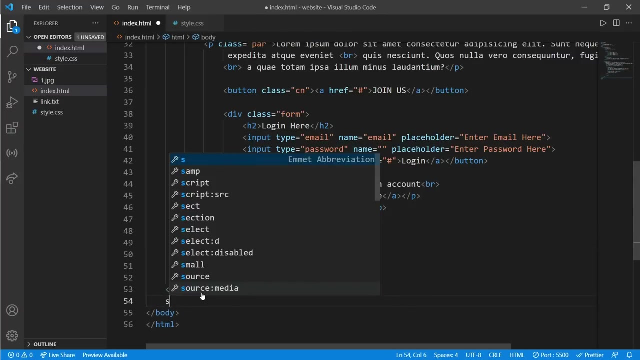 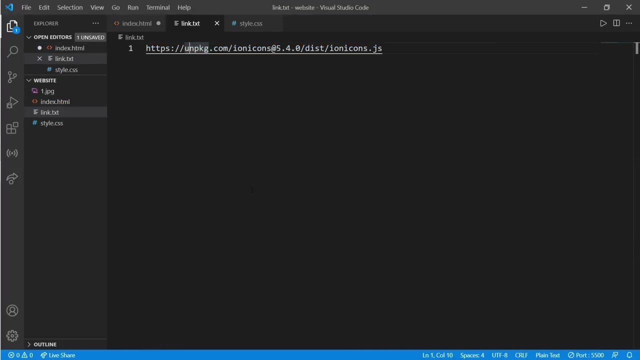 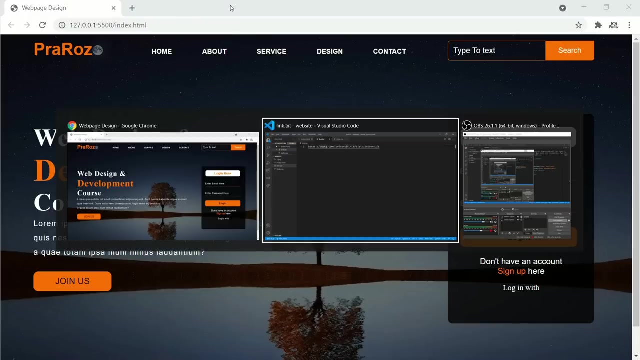 paragraph tag is up. keep it down. now it will work. okay, you just want an sign up to be highlight, so put closing anchor tag over there. okay, it looks more good. you know, we put our script source. click in the link which is in the description and copy their URL. copy the URL and paste it inside the quotation mark. okay. 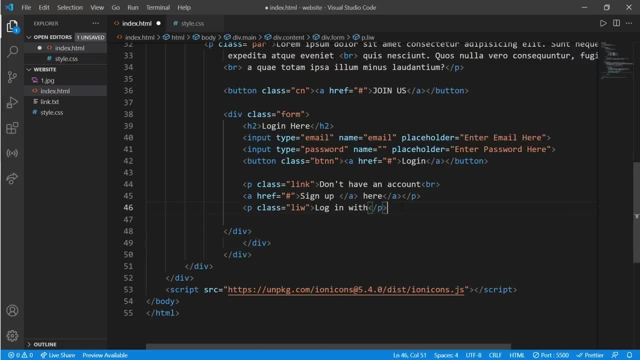 now we will create another deep, that is for our icon anchor tag. I own icon name equals to logo Facebook. okay, here we have our logo of Facebook and copy: similarly, we put Instagram login with Twitter, Google and Skype. okay, here we have our five logo and icons, okay. 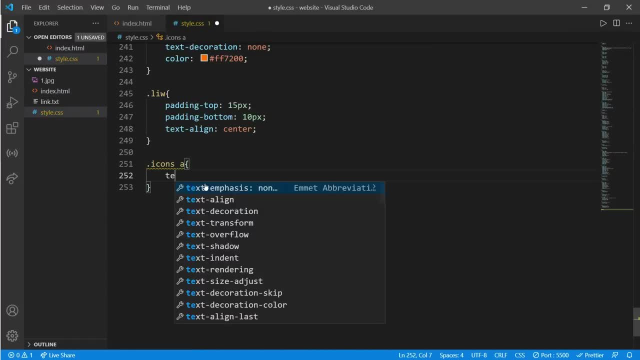 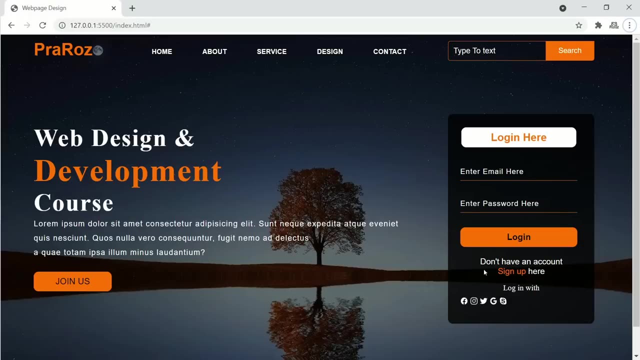 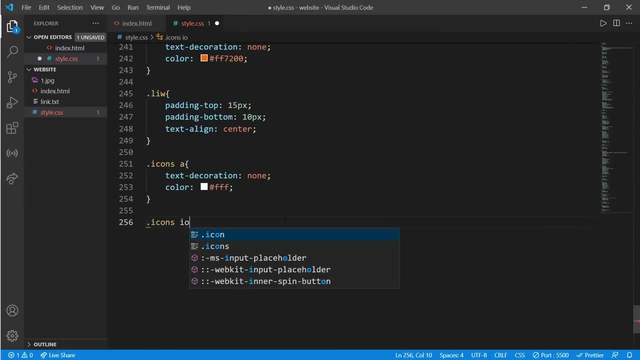 dot icons. text decoration on color would be white. yeah, here is our white color icons. and that icon, I an icon. we put color white, right and then font size of 30 pixel. and Monza icon icon: we put color white, white and then font size of 30 pixel. and. 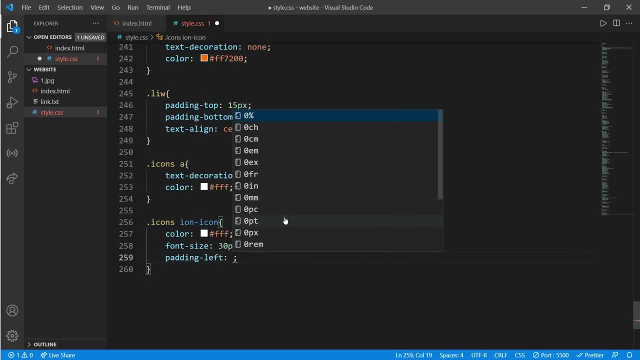 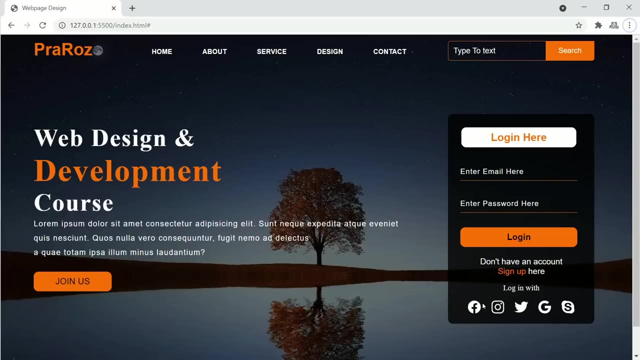 padding dialogue. we just missed set in theек ainda. okay, this is the code where you paste in text as code in font size 4 and next things like as to icon number, sortings from one icon to one key and Definition. you just display left would be 14 pixel and padding top would be 5 pixel. okay, it looks more good.